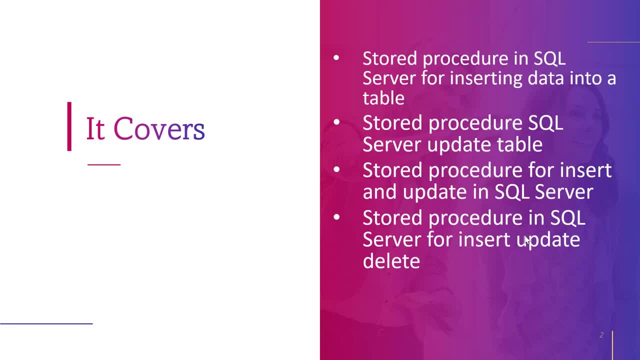 discuss how we can create a stored procedure to update the data of the table, and then we will create a stored procedure for both the operations- insert as well as update. and in the last we will discuss how we can create a stored procedure which will insert, update as well as delete some. 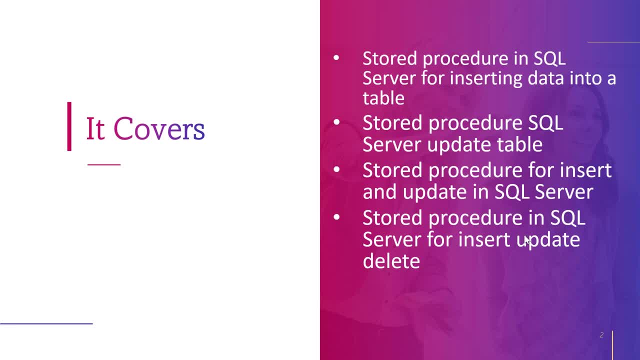 records. now, before we start off, i would like to tell you that we regularly come up with these type of tutorials, so if you really like our tutorial, please subscribe to our youtube channel now without any further delay. let's jump to the very first topic and let us discuss how we can. 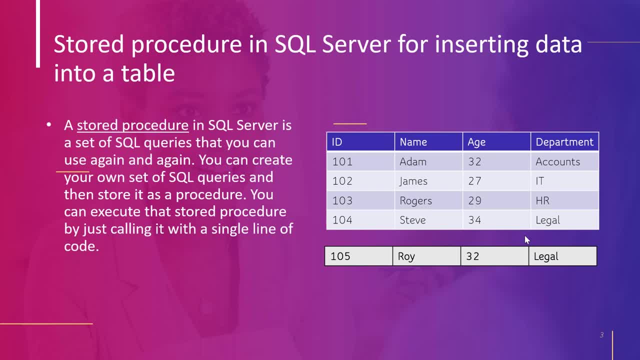 create a stored procedure in sql server for inserting some data into a table. now, what is a stored procedure? basically, stored procedure is a set of sql queries that we can use again and again. we can create our own set of sql queries and then store it in a procedure, so a 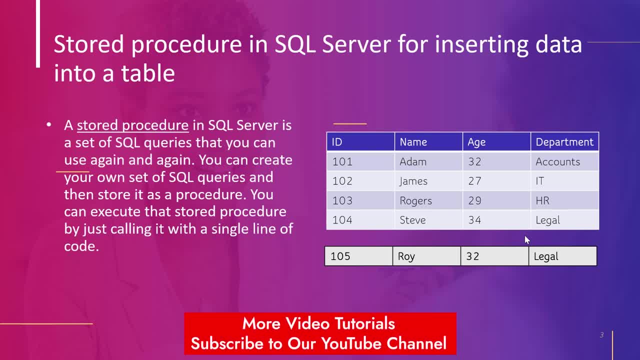 stored procedure is nothing but a place where we can store set of sql queries. now we can execute a stored procedure just by calling its name. what will happen? we can use a stored procedure to store multiple sql statements and then we need to just call the procedure name to execute all those. 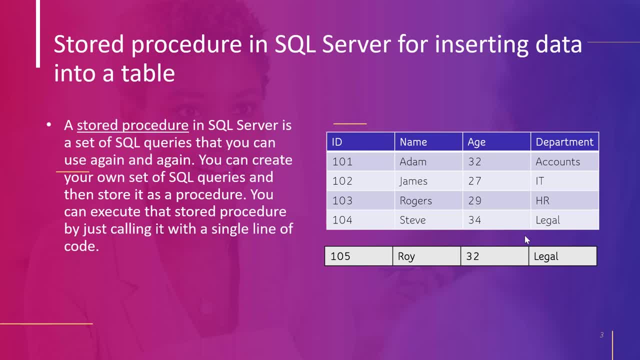 queries at once. now, to understand how we can create a stored procedure for inserting data into a table, we will implement one example. so what we will do in this example? first we will create a table. then we will insert some data into the table. after this we will create. 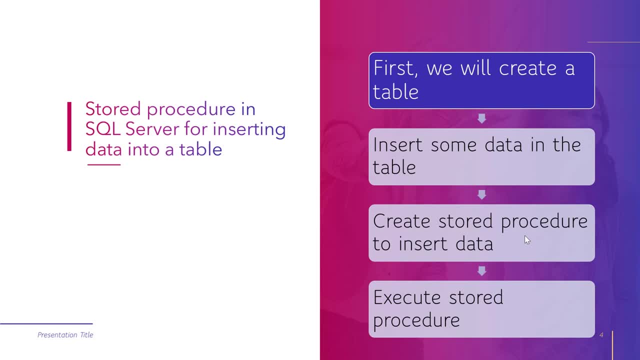 a stored procedure which will implement one insert statement and with the help of the stored procedure, we will insert some data into the table. now how we can do that: we need to call the procedure and with this stored procedure, we need to use multiple input parameters so that we can pass input values. 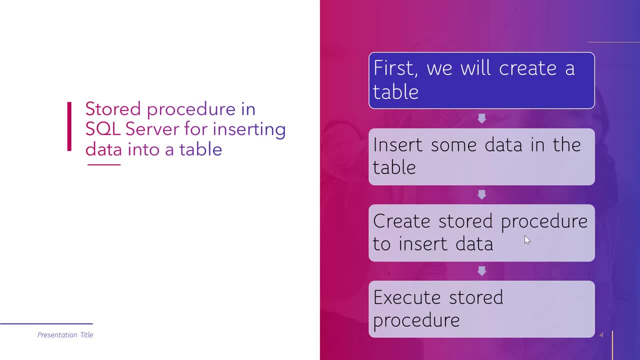 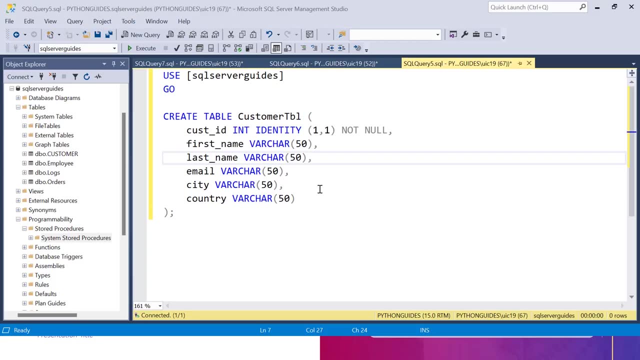 to the procedure, and procedure will pass that values in the insert statement so that we can insert that data into the table. now let's execute this example. so here i have opened my sql server management studio. in this i am using create table statement to create a table with six columns. so 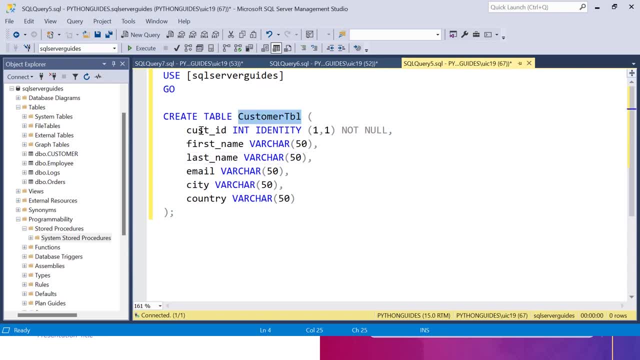 the name of the table is customer table. after this we have defined six columns. so very first column is this cust underscore id, which represents customer id, and it is an auto increment column which is of integer data type. then we have defined a table which is of integer data type. then we have: 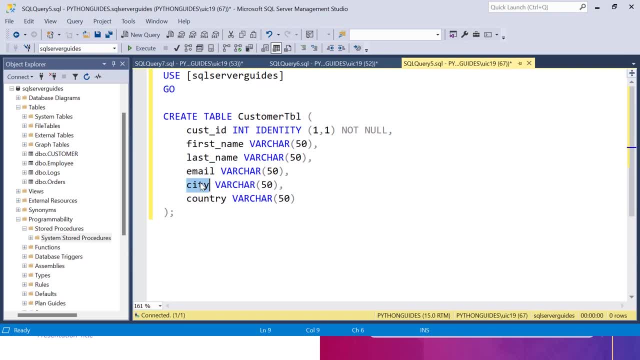 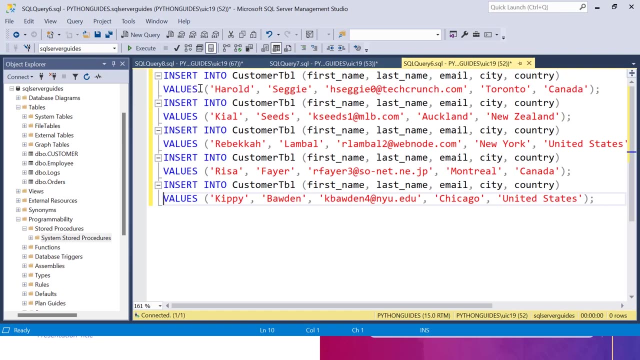 defined first name, last name, email city and in the last we have defined country. so if i execute this code block, it will create a table with name- customer table, tbl. now the next step is to insert some data into the table. so here i am using multiple insert into statements so that 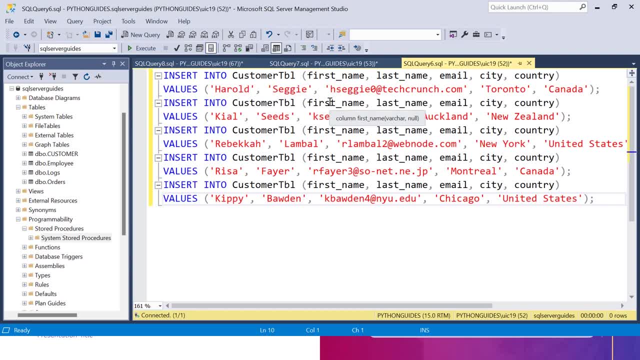 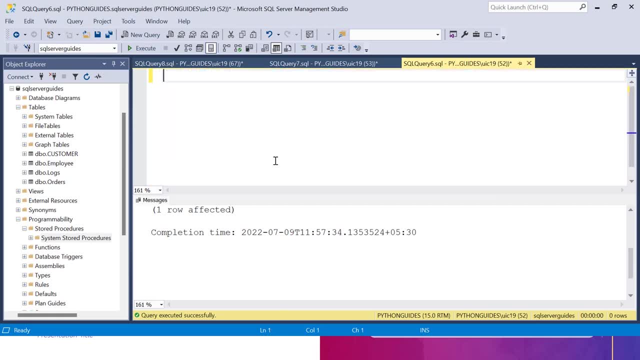 we can insert some data here. i am inserting five rows of data in the table. let me execute this as well. so here you can see. all these statements has been executed. now let's look at the table, the data of the table. so for this i will simply use the select statement. let me execute this and. 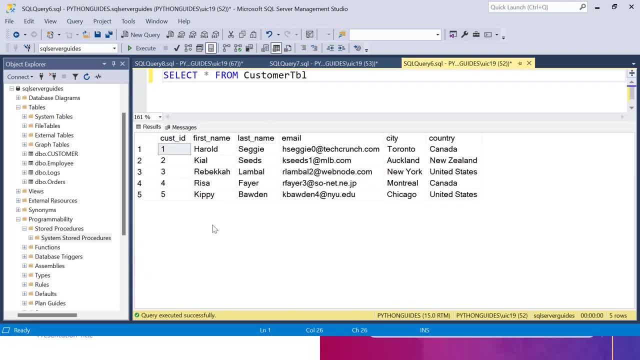 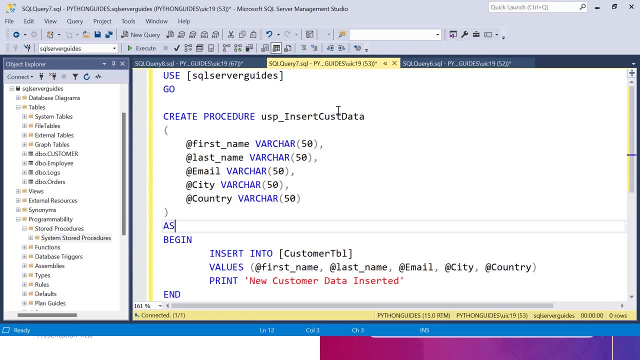 here you can see the data. so this table consists five rows of data. now let's move to the actual step, where we will create a stored procedure. so here you can see the code for creating a stored procedure. so what we are doing in this code? first, we are specifying that we are using this database. 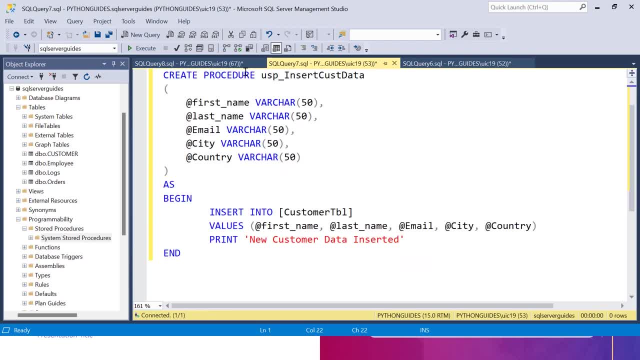 the name of this database is sql server guides. after this, we are using a create procedure statement to define a stored procedure, and this is the name of the stored procedure, which is usp. underscore: insert: cust data. the usp here is a naming convention, so it it represents. 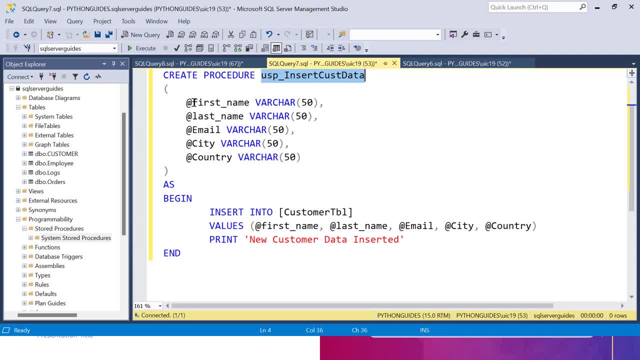 user defined stored procedure and after this we are using brackets and within the brackets we have defined five input parameters. so very first parameter is first underscore name, then we have last name, then we have email, city and country. so in this way we have defined five input parameters. 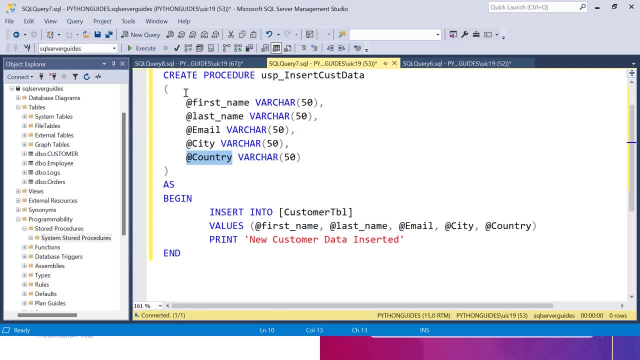 we did not define the input parameter for id because we have set it as auto increment. after this, we are using the as keyword and then we have defined this begin and end block. now, within this begin and end block, we are simply using an insert into statement, so we have specified: insert into then the name of the table, which is: 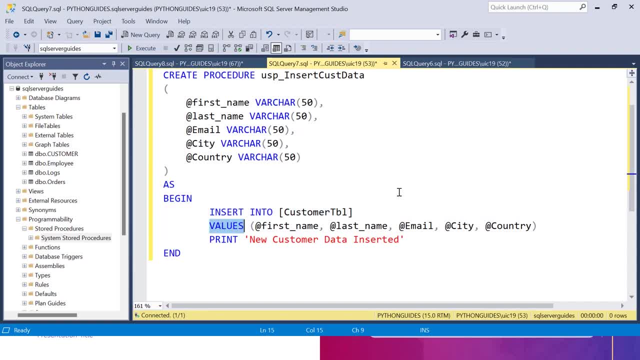 customer table, then the values keyword and then, and within the brackets, we need to pass the input parameter. so, with the help of first underscore name, we will set the first name with last name. we will specify the last name with email. we will set the email in this way. we are inserting: 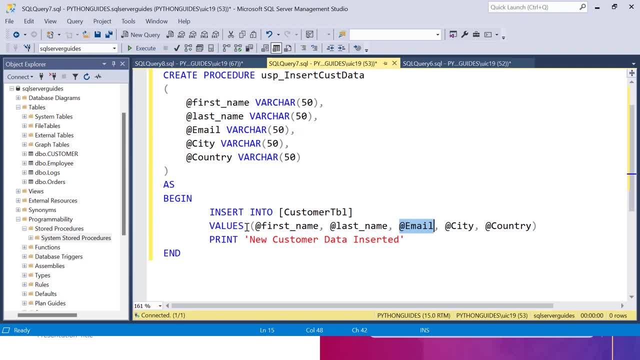 one single record in the customer table and once this insert statement has been executed, we will execute one print statement and this print statement will print this new customer data inserted. let me execute this code block and here you can see: our store procedure has been created successfully. now let's start using it. so now let's see how we can execute this store procedure. now to 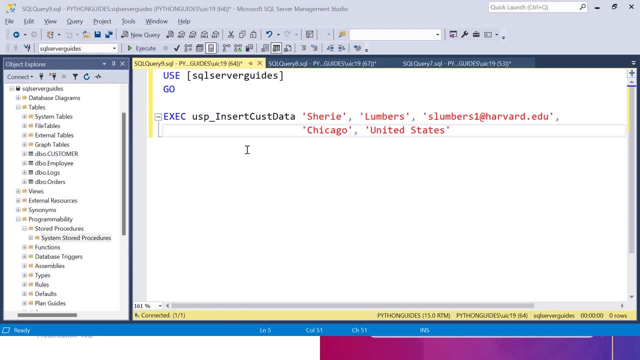 execute the store procedure. we either use execute keyword or we use the short form exec for execute. then we need to specify the name of the store procedure that we want to execute. after that we need to specify the name of the input parameters that we want to pass. so here we have passed five. 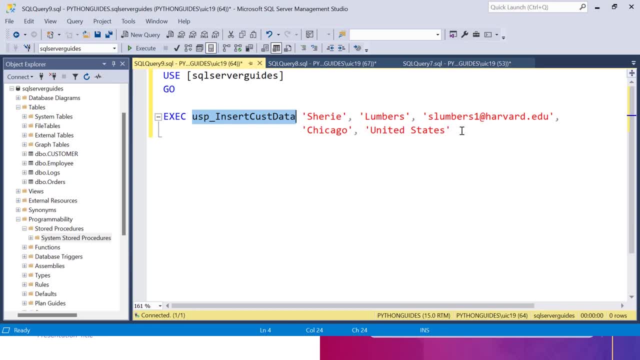 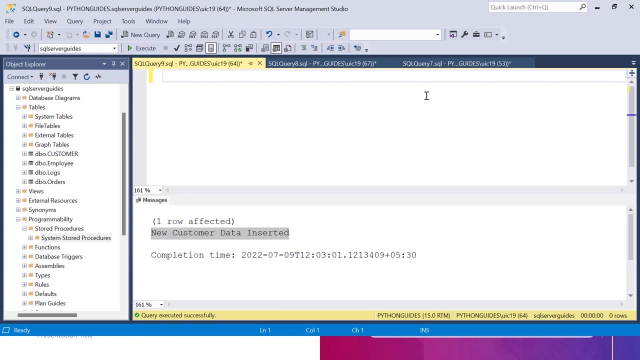 input parameter values. all these parameter values are of string type. now let me execute this, and here you can see it has returned this thing: new customer data inserted, which means our insert statement has been executed successfully and this record has been inserted in the customer table. now let's check it by using the select statement. so here is my select statement: select star from. 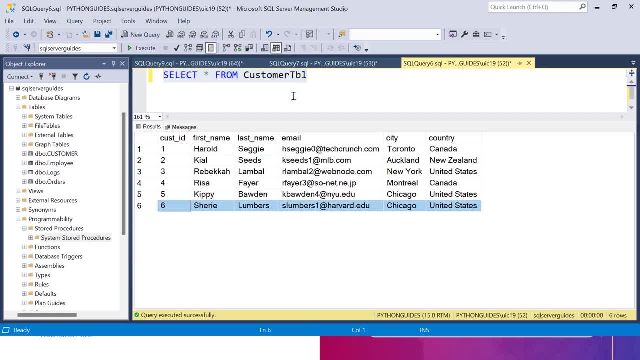 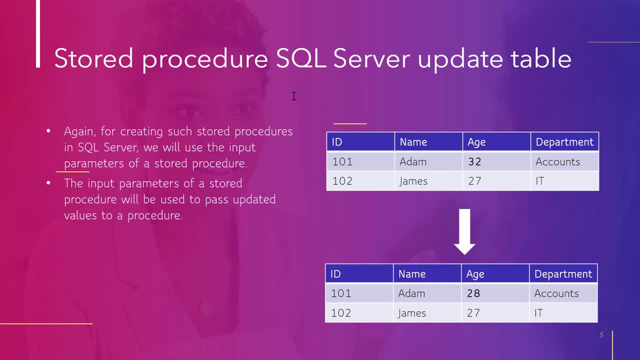 customer table and here you can see, six record has been added. so with this we have understood how we can create a stored procedure and how we can insert data using it. now let's move forward and let's discuss how we can create a stored procedure for update operation on our table and again for creating a stored 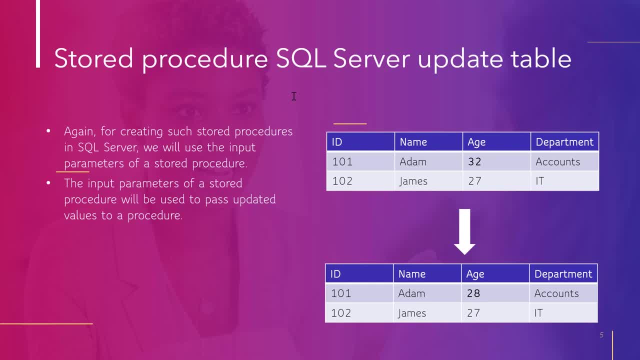 procedure in sql server, we will use input parameters, and input parameters of stored procedure will be used to pass the updated value. so, just like we have created the stored procedure for insert operation, in the same way we will create a stored procedure. we will keep some input parameters so that we can pass updated values and, instead of using the insert, 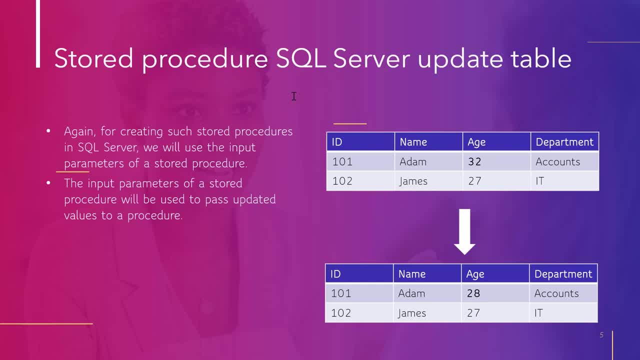 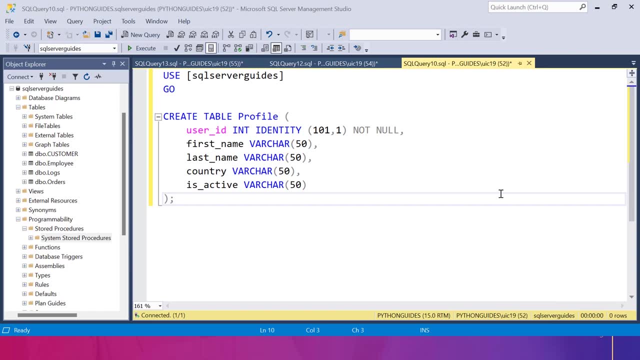 into statement. we will use update statement and update data, update data of the table. so let us discuss how we can do that with the help of an example. now for this execution also in sql server, we will use the same approach. so first we will create a table and in this case we will create: 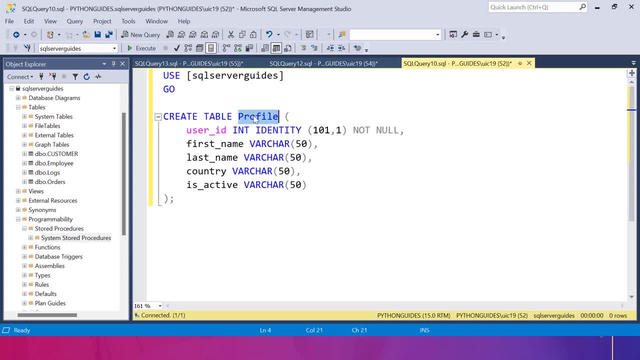 a table named profile and in this we have specified five columns. so very first column of this profile table is user underscore id, which is an auto increment integer type column. then we have specified first name, last name, country, and we have specified another column which is is active. if i execute: 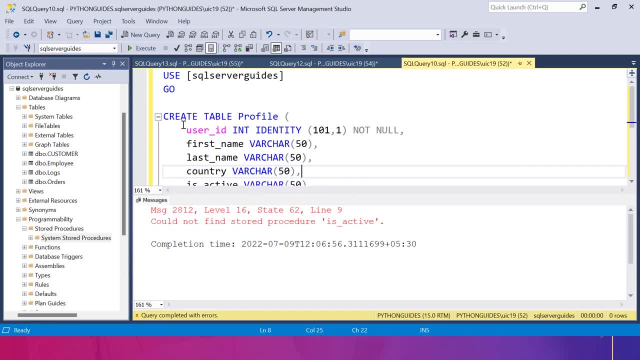 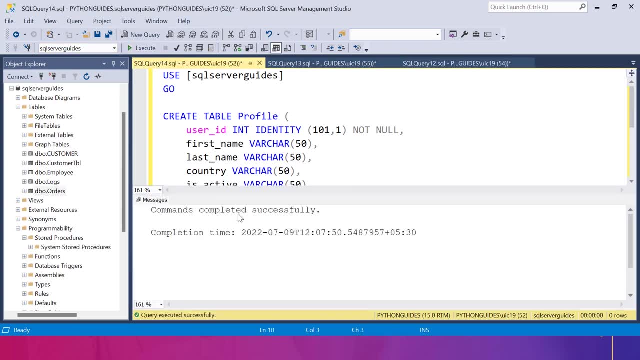 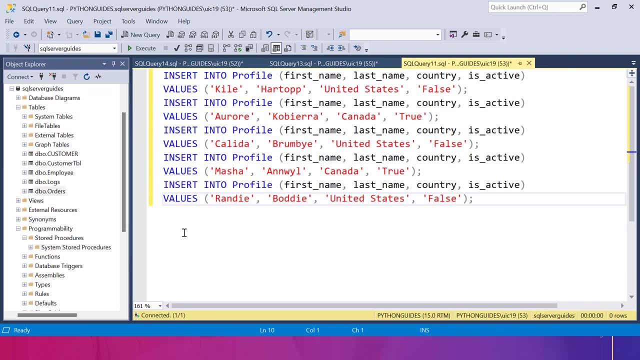 this code block. i am extremely sorry. i have selected is exactly that's why it has returned this error. now let me click somewhere else and then execute this now. now, if i execute this code block here, you can see a command has been completed successfully. this means our table has been created. once the table has been created, so the next step that we 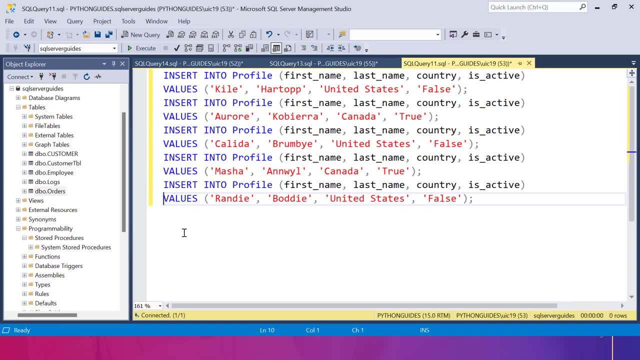 are going to execute is to insert some data into the table. so here we are using insert into statement to insert five records. so by executing this code block, we have successfully inserted five rows in the profile table. let's check it with the help of a select statement. 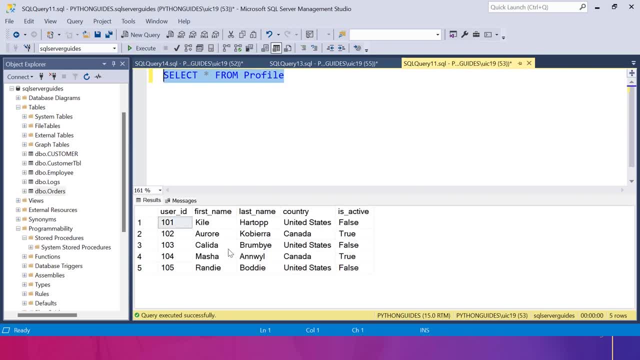 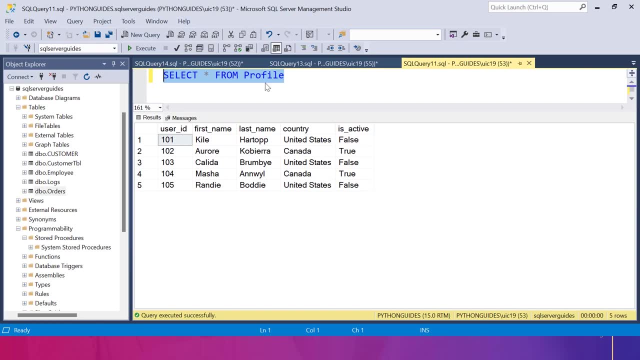 so i will write select and let me execute this select statement. and here you can see five records has been there in this table. now let's move to the actual step where we will create a stored procedure, and here on the screen you can see the sql code first, 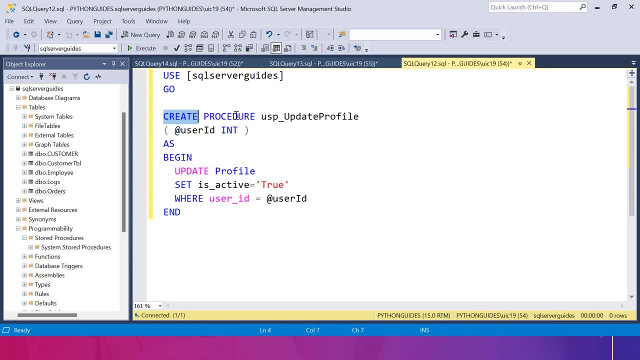 we have a stored procedure. so first we are using this create procedure command: create a stored procedure with this name, which is usb underscore- update profile, and then we have specified one input parameter, which is user id, which is of integer data type, and then we have defined as keyword and within that we have specified the beginning and block. 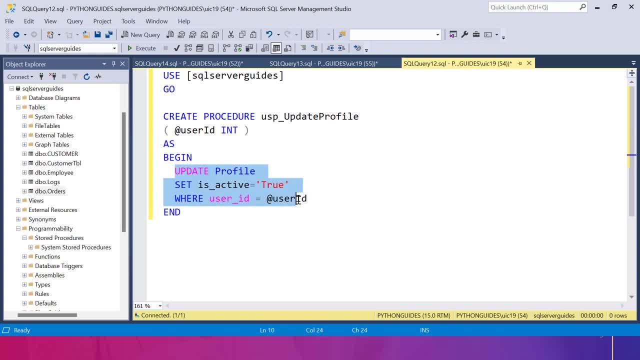 now our update statement will be placed within this beginning and block. and what we are doing with this update statement? we are simply updating the profile data and we are going to create table and we are setting the value of is active column to true where the user id is the one which 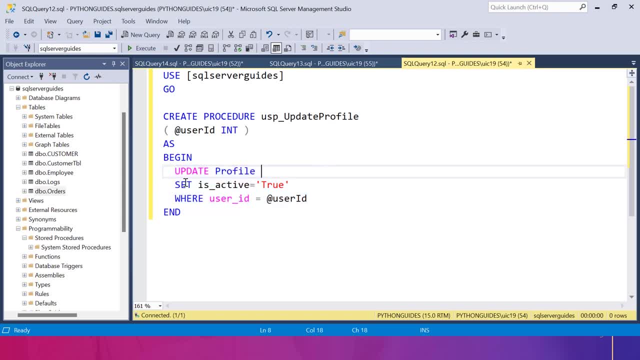 we have specified as an input parameter. so that's why we have used this statement- update profile- to specify the profile table that we are going to update it. then we are setting the value using the set keyword of this is active column to true, where user underscore id is the user id that we 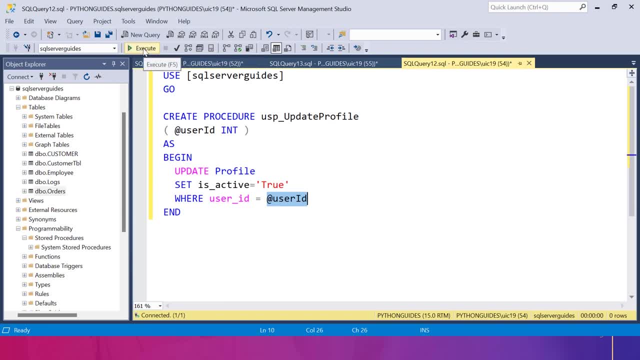 have specified as an input parameter. let me execute this code block. and. extremely sorry, i have selected user underscore id. that's why it has returned this error. let me execute it once again. and with this we have created our stored procedure. now let us understand how we can use this stored. 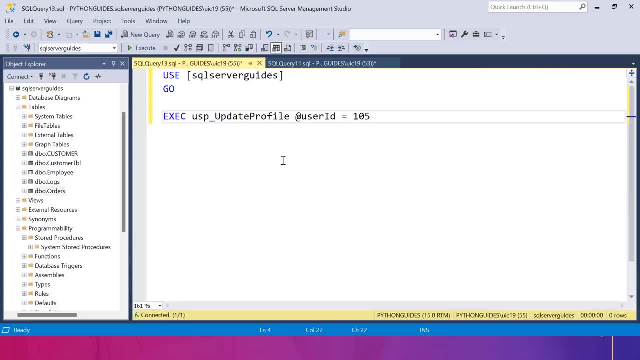 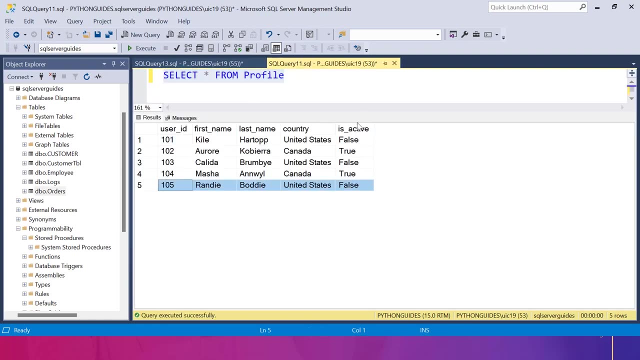 procedure to update the data of the table. so here you can see: we are executing this update profile stored procedure using the execute keyword and we have specified the value of user id as 105. so if i show you the table, at 105, we have this record and here you can see the value for is active. for this record is false. what so? what we? 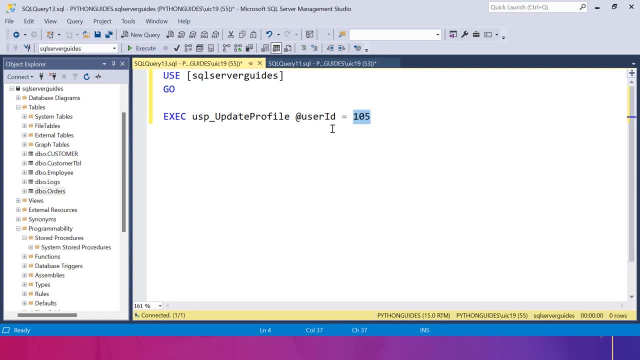 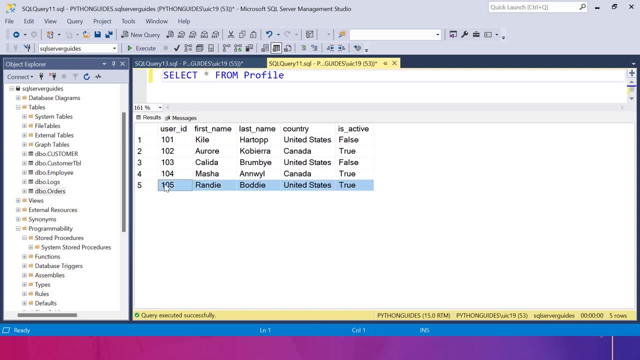 are going to do? we are going to update its value of is active from false to true using this stored procedure. so let me execute this code block and it has returned this thing. one row affected if i come back and if i execute this next statement again, and this time you can see for record 105. 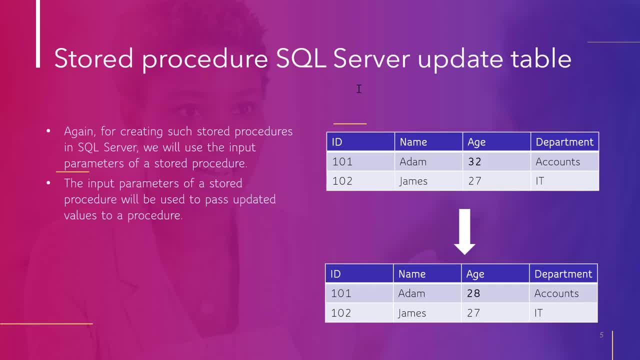 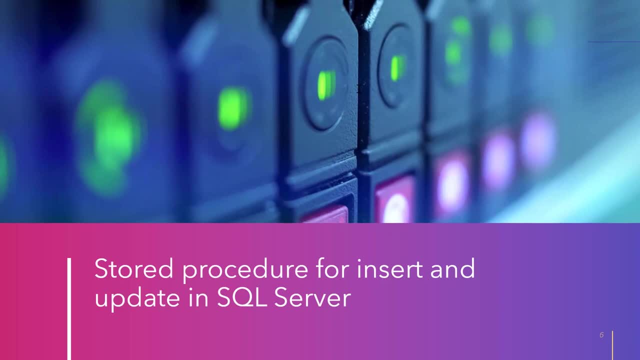 the is active value is true. so with this, i hope you all understand how we can create a stored procedure, update data of a table. and now let's move forward and understand how we can create a stored procedure which can execute both of these tasks at once. so we will understand how we can create a stored procedure that can insert as: 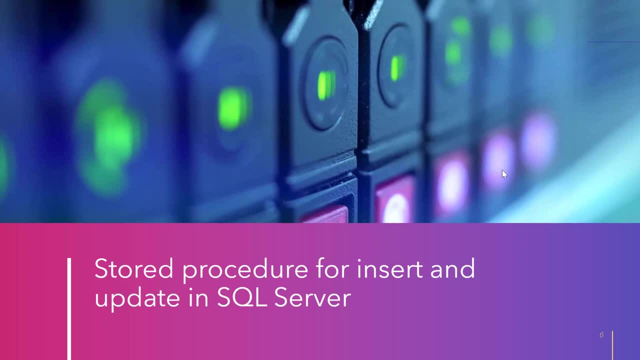 well as update data into our table. so, for this task, what we will do, we will create a store procedure which will implement both insert as well as update statement. now, to pass data into the stored procedure, we need to use input parameters. so let us understand how we can do this implementation with the help of an example. 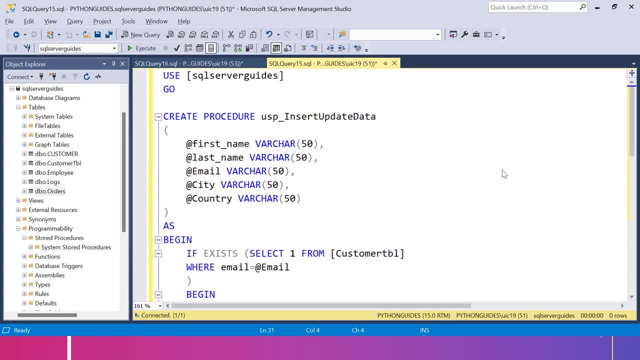 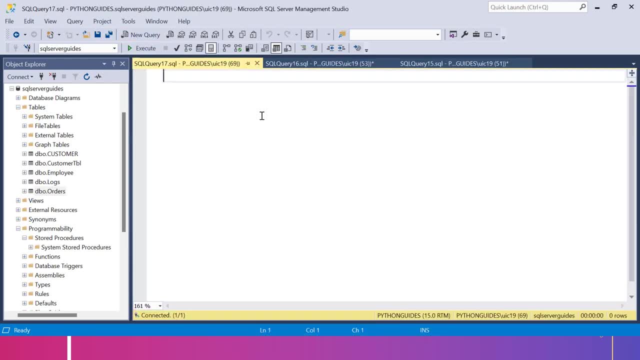 and here you can see we have created one stored procedure. now, what we are going to do, we are going to use the customer table for this implementation. so if i show you the select statement again, so here you can see the customer table which we have created in the very first. 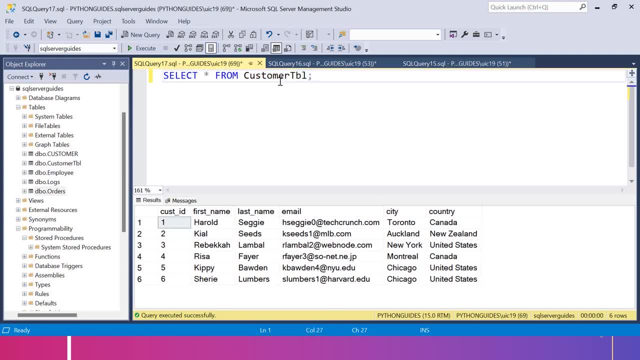 example now. currently it has six records. so what i will do? i will create a stored procedure which will take input parameters. it will take values as input and then it will check whether the record is present in the customer table or not. now, if the record is already present, then it will update. 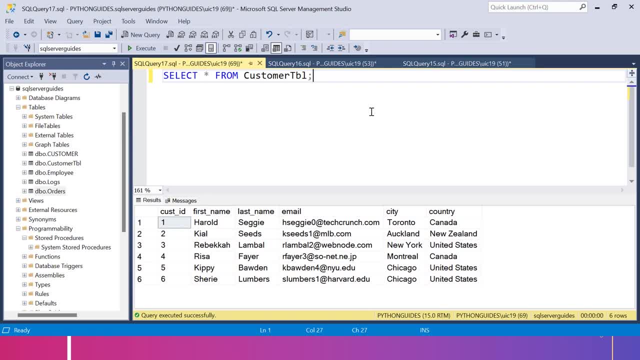 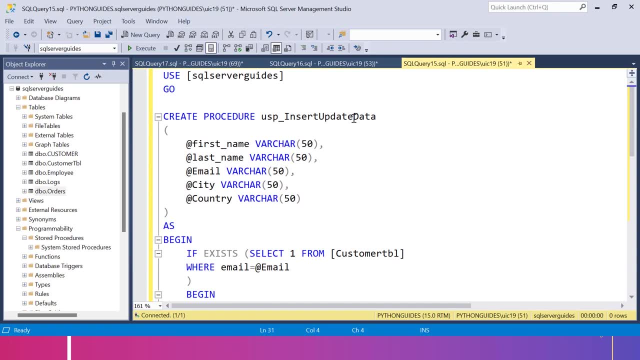 that record, and if the record does not present, then in that case it will insert that record. so let me show you this sql query for this example. here again we are using the create procedure statement to create a stored procedure with name insert, update data. then we have specified five input parameters: first name, last name, email city and. 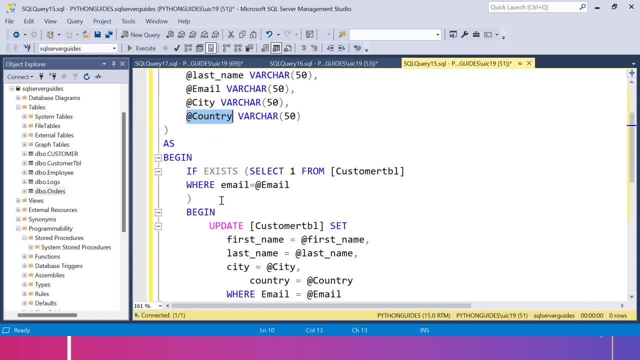 again country, then we have specified the begin end block and, within the begin end block, what we are going to do. we are going to use the email and we will check whether the record or the email that we have passed as an input already exists in the customer table or not. as we all know, email is such 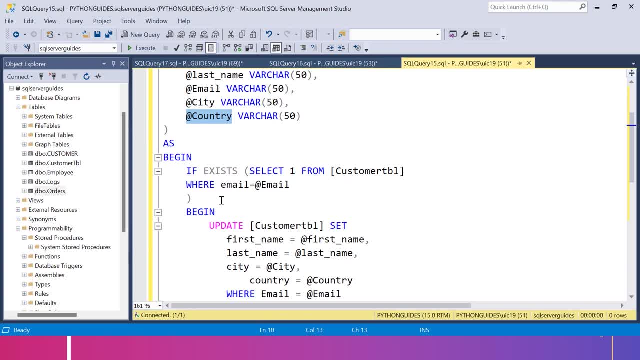 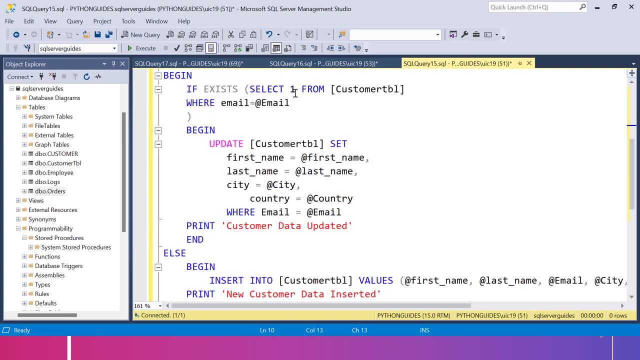 type of field which will be unique for each user, so we can use this field to check the existence of a record. so here you can see, we are using if exist statement and within that we are using the select statement to check whether the email already exists in the table or not. the email already exists, it means we need to. 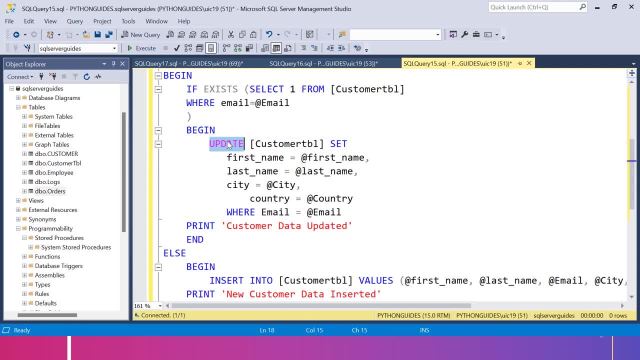 update that particular record. so we will use the update statement on the customer table. let me change it because it is capital t, and then we will use the set keyword to set the value for each column as specified in the input parameter. so we will set the first name as the. 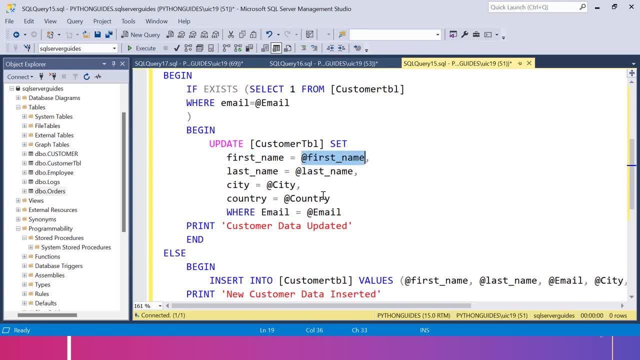 first name that we have passed as an input parameters, and we will do the same for all the records, except for email, because we are using email to check the existence of that particular record. now, once this update statement has been executed, we will print this string, that is. 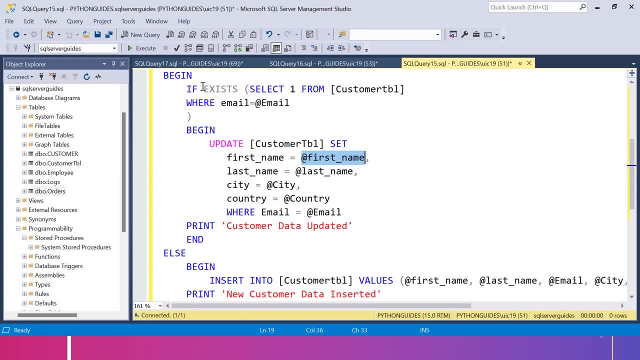 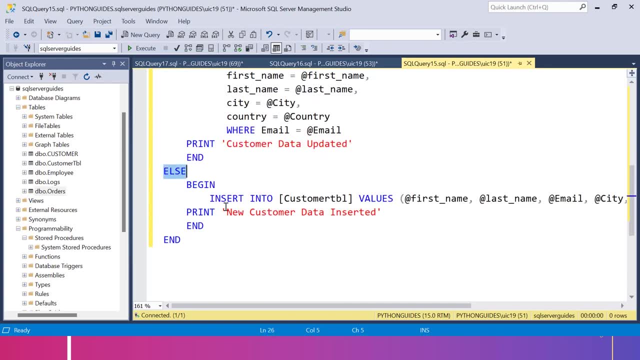 customer data updated. now, in the starting of this begin block, we have used this if statement to counter this. we will also have the one else statement where we will use the insert into statement. what if the email does not exist in the table? then in that case we need to insert record into the table. 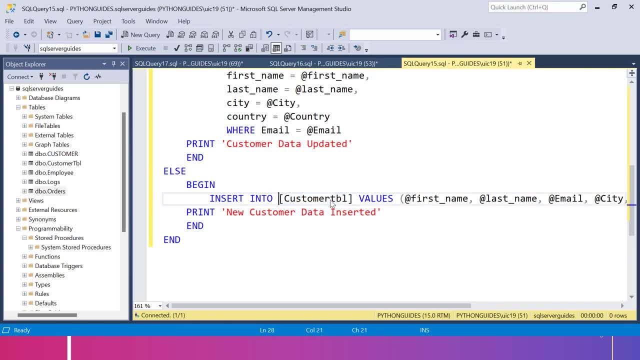 so we will use insert into statement on this customer table. and again here in the customer table, t is capital, so let me modify it, and then we need to specify the values and once this insert statement has been executed, this string will be printed out, that is, new customer data inserted. so 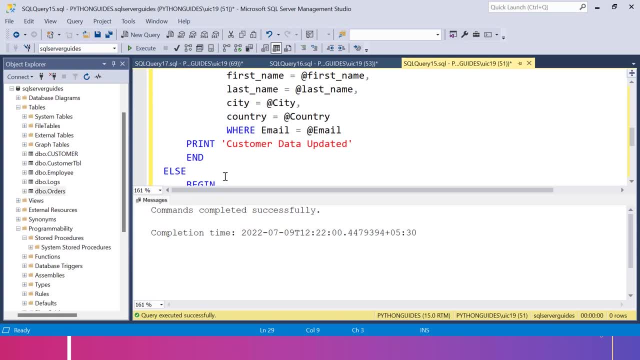 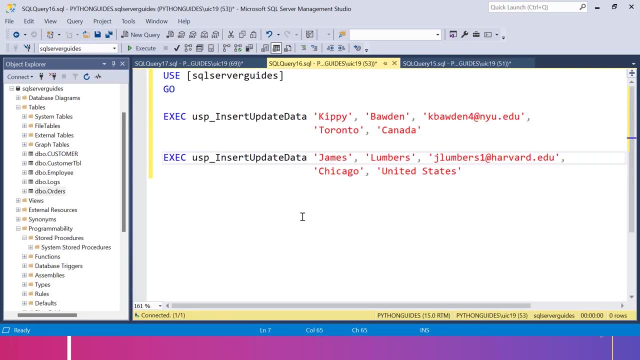 now let me execute this code block. and here you can see, the stored procedure has been created successfully. now let's understand how we can use this stored procedure. now. here you can see the sql query for execution of this stored procedure. so what we are going to do? first, we are using this execute statement. 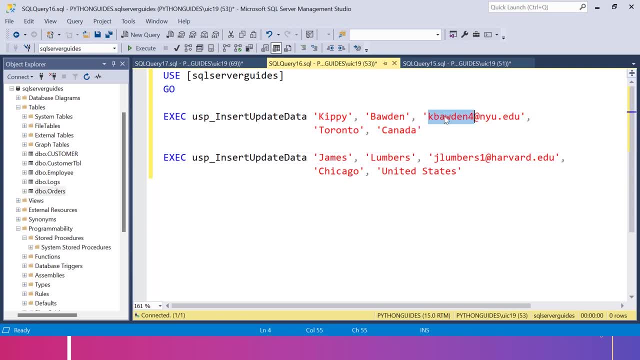 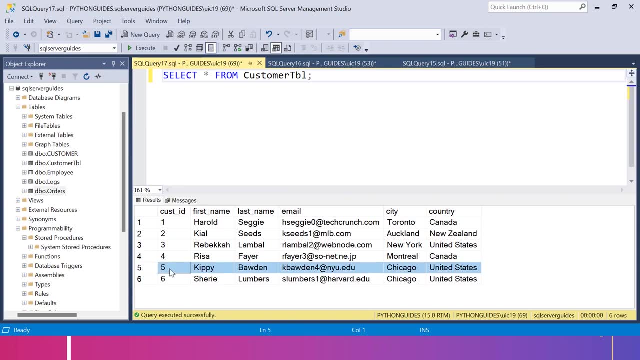 to update data of the customer table. if you look closely to this email address, this email address is already there in our table, which is at index 5, so customer id 5, and we have this email address, which means it is already there in our table. so what we are modifying? 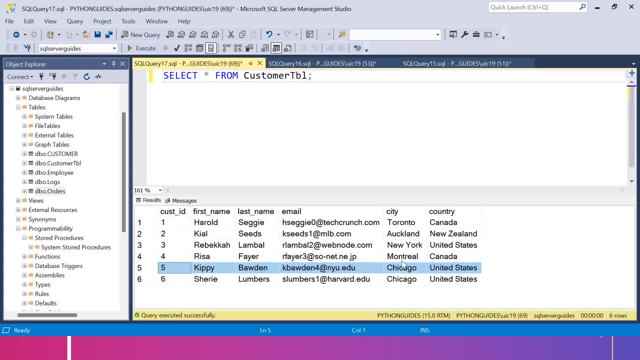 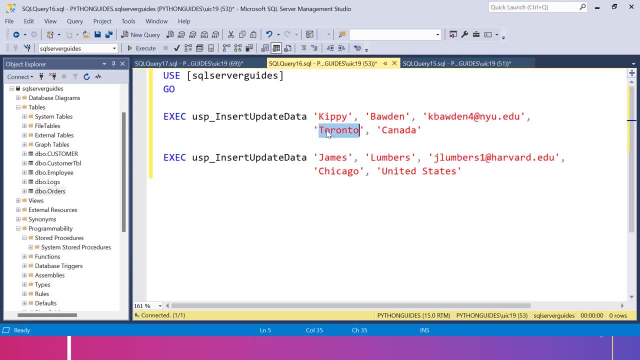 we are modifying the city and the country. so for this record the city is chicago and the country is united states. but with this stored procedure we have passed city as toronto and country as canada. so this is how we are going to use the update operation from the stored procedure and after. 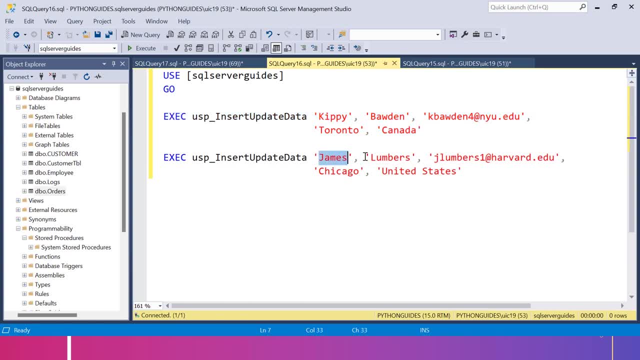 that we have passed one unique record. name of this record is james. here you can see one unique email user. so very first execution statement will update the record and the second execution statement will insert the record in the customer table. so let me execute this code block and here you can see: 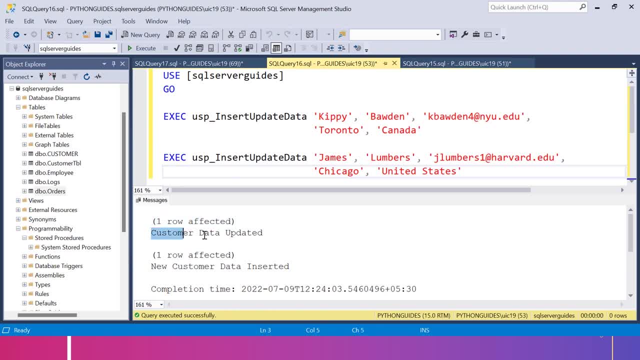 it has returned one row affected for the first store procedure and it has written this thing: table customer data updated and then it has again updated the one record and it has returned new customer data inserted. now, if i show you the select statement, let me execute it back. 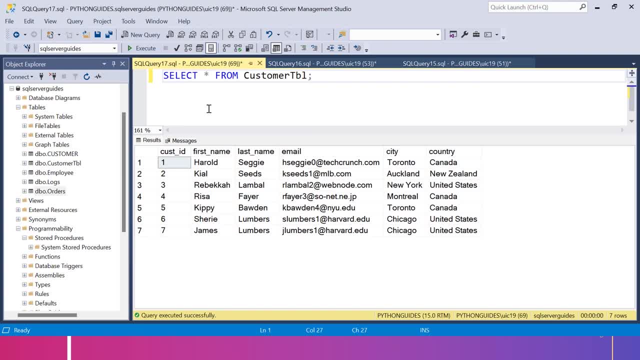 and here you can see earlier, we have six records. now, after the execution of the store procedure, we have seven records now. the james record has been added in the very last and for uh, customer id 5, where we updated the city and country, so it has toronto now and the country is canada. 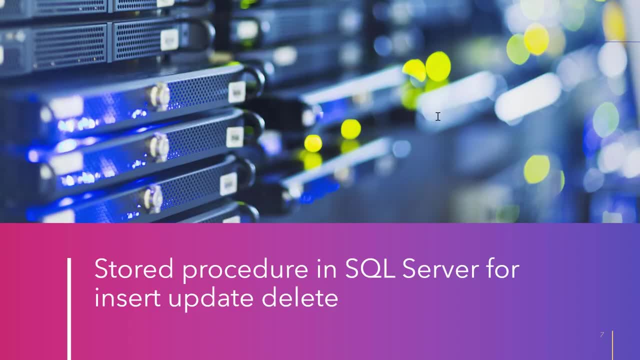 now let's move forward and let's discuss how we can create a stored procedure for implementing insert, update and as well as delete operation on a table. now i hope you all understand how we can execute insert as well as update statement, but how we can implement delete statement, let's discuss. 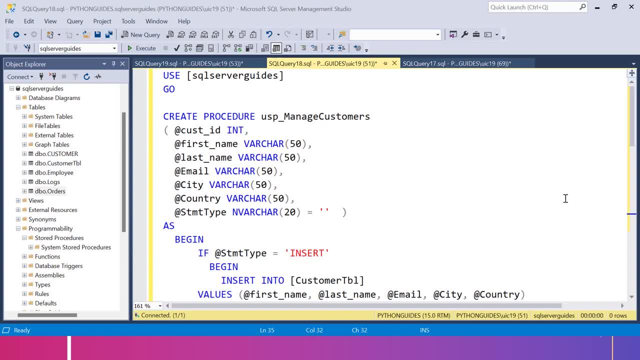 that with the help of an example. now again, for this execution we are going to use the same customer table, and here you can see the code for the stored procedure. here we are creating a stored procedure with this name: usb underscore- manage customers, and with this we have specified seven. 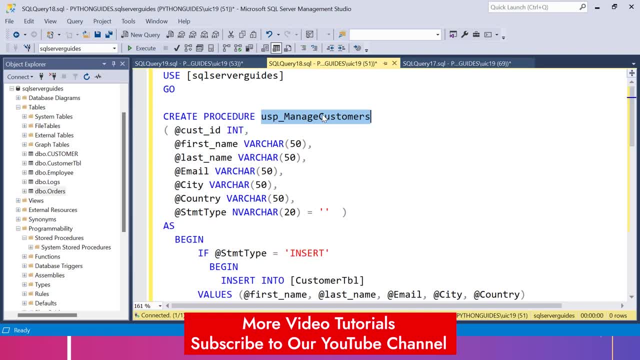 input parameter. very first parameter is customer id. then we have first name, last name, email city. last we have this statement type. now this statement type input parameter will be used to recognize whether we want to implement the insert statement, update statement or delete statement. now, after this, we have specified the ask keyword and then we have specified the begin, end, block and within: 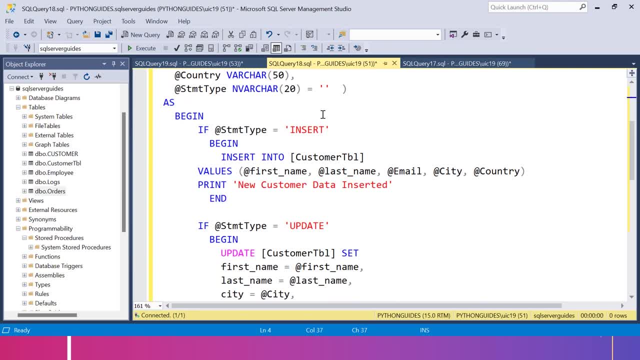 the begin end block. first we are checking if the statement type is insert. so here we are using the insert statement. so if the statement type is insert, then we are going to implement insert into statement on the customer table and then we will use the insert statement and then we will use. 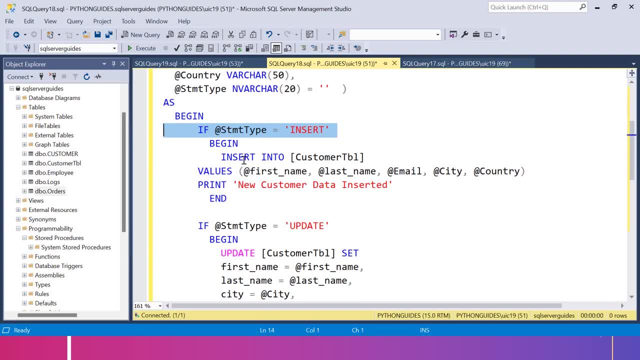 all the input parameters to insert data into the table and then we will use the insert into statement to insert all the input parameters to insert data into the table and once this insert statement has been executed, we will use the print statement to print this string: new customer data. 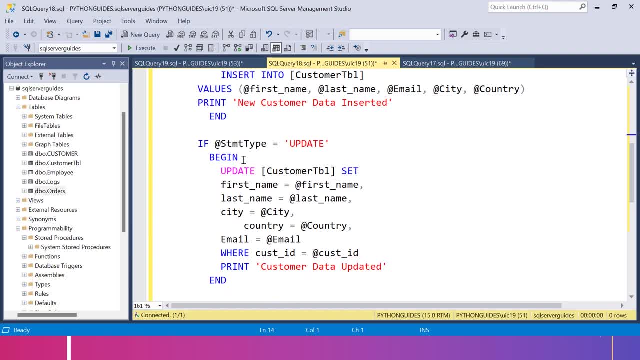 inserted. after this, we are again using the if statement to check whether the statement type is update. so if the statement type is update, we are going to implement the update statement on the customer table and we will update all the records here. to update the record, we are going to use the customer id, which is a unique for every. 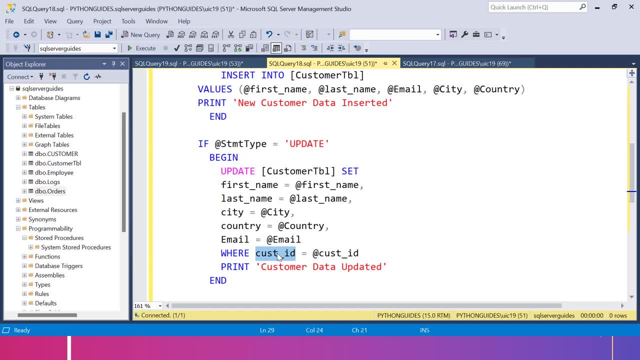 customer. so we will use the customer id in our where clause and once this update statement has been executed, we are going to print this string stating customer data updated and after this we are again using else if statement to check whether the statement type is delete. so if the statement 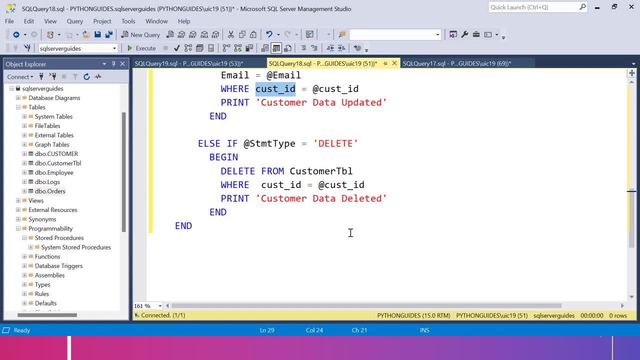 type is delete, we are going to execute the delete statement, so we will use delete from then the name of the table, which is customer table, and then we are using the customer id as our to delete data from this customer table and once this delete statement has been executed, we will use the print. 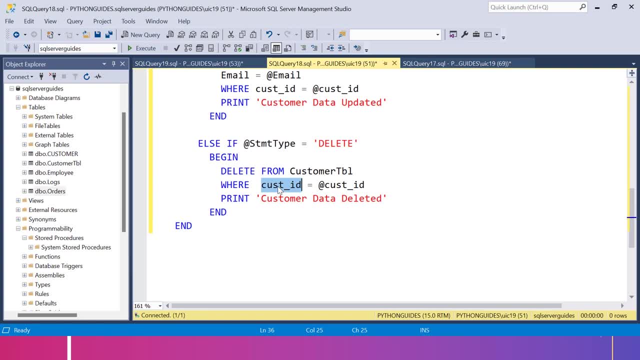 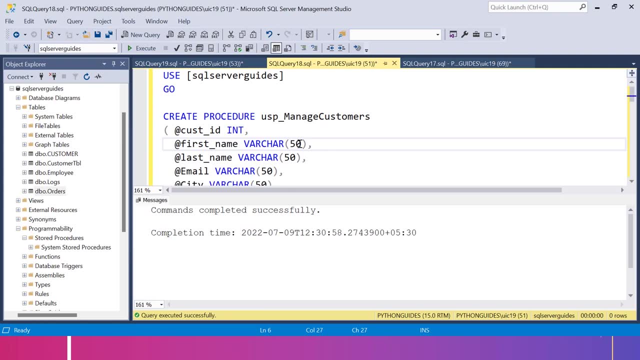 statement to print the string on the screen which is customer data deleted, so that we get to know which statement has been executed. let me execute this code block and with this we have successfully created our stored procedure. now let's discuss how we can use this. now, here you can see i am. 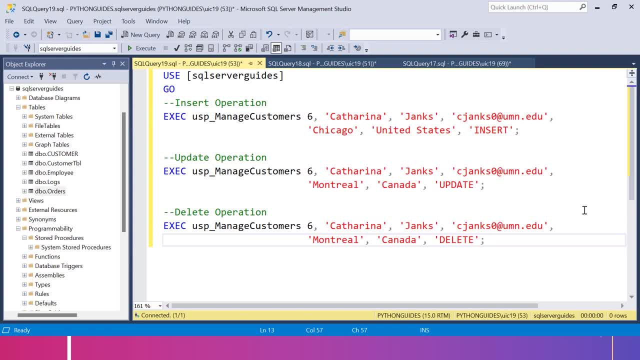 going to pass the insert parameter three times. very first, execution statement is to insert data. and here you can see, in the last i have passed insert as my input parameter to specify that we are going to implement the insert statement. now here one thing we need to, or we can say we need: 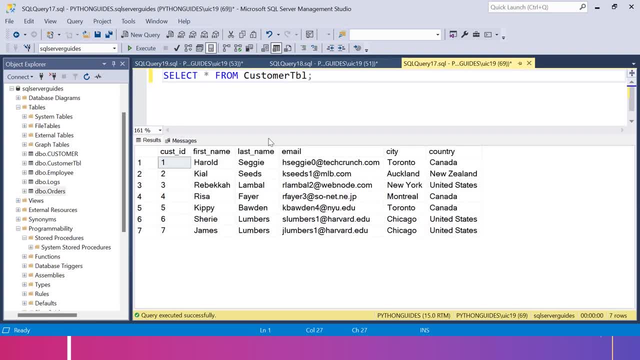 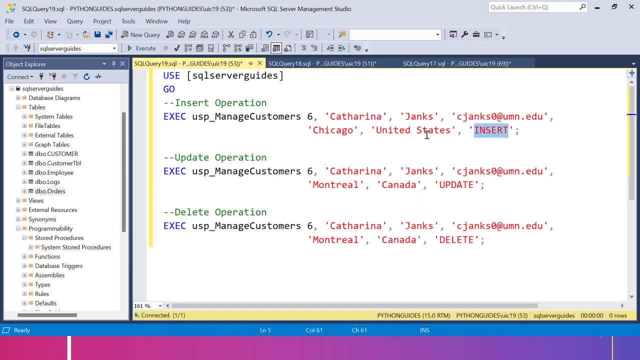 to be careful with. if we look into the customer table, may execute it. if we look into the customer table here you can see there are seven customer ids. now while passing input parameters we need to be pass unique customer id, so i will pass 8 for that. so for the customer id would be 8, the name. 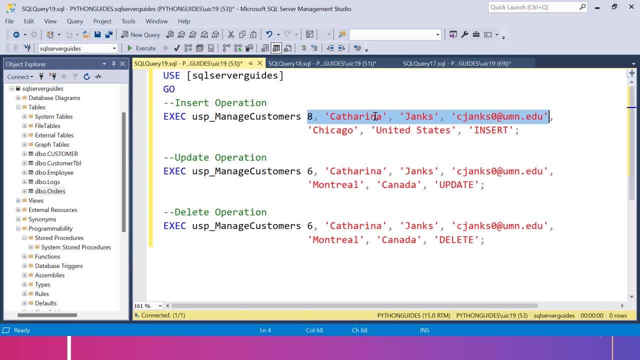 will be katharina janks and this will be email address, then the city, then the country and then we are specifying that the statement type is insert. let me select this and execute, and here you can see macro affected: new customer data inserted. with this, we have implemented insert. 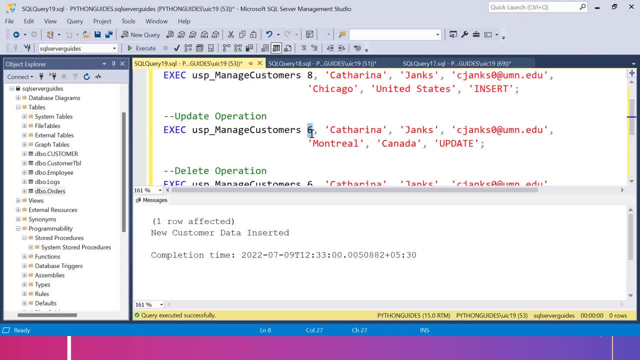 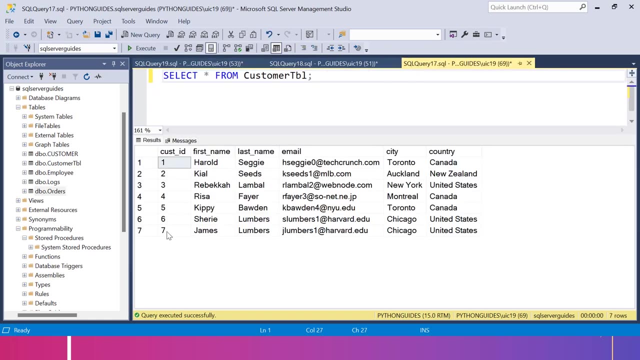 operation. let's move forward, and this time i will keep the ids 6 only, and i have specified this thing, that we are going to implement the update statement. so again, i will select it and execute it, and here you can see one row affected and customer data updated. now earlier, at number six, we have this record, which is sherry lumbers. 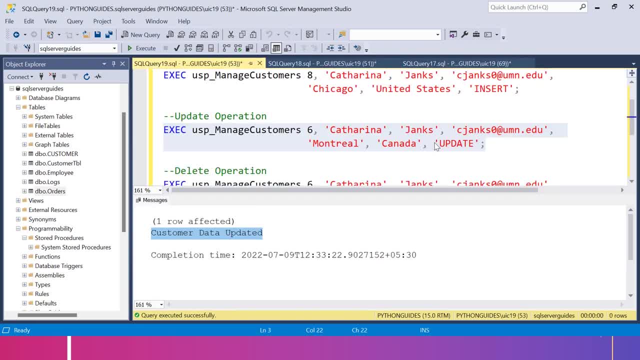 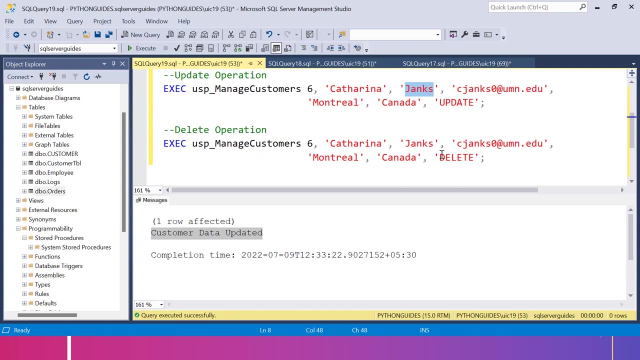 is the last name. sherry is the first name, but while execution of the update statement, we have specified the first name as katharina. his last name is jenks, so this will update the user record given at user id 6 and again in the last. we are using the delete operation on. 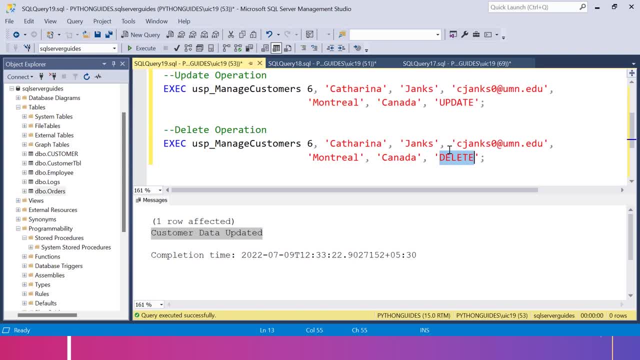 the stored procedure. that's why we have specified leap as our statement type and again, we are going to delete the record which is given at user id 6.. so before executing this delete operation, let me show you the customer table again, and here you can see, this is our table. we have inserted. 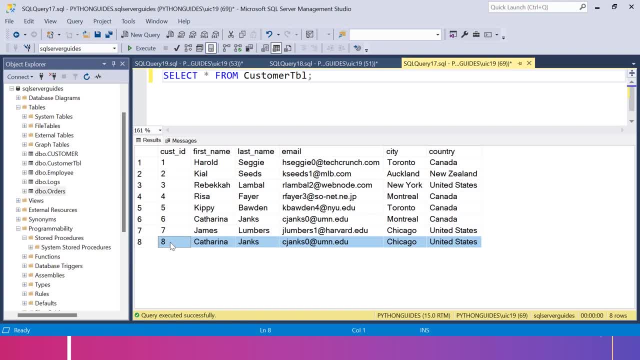 one record at index eight. so customer id eight is katharina janks. this is the email address, city is chicago and the country is united states. and then we have updated the record which is at a user id six. so earlier it was something else, now it is katharina janks and 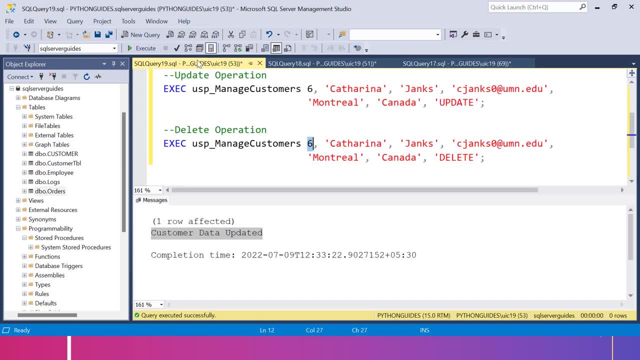 here you can see the country and city, for this record is different now. next we are going to implement the delete operation. so let me execute this sql query and you can see customer data deleted. now let's come back to the select statement and again execute it, and here you can see the